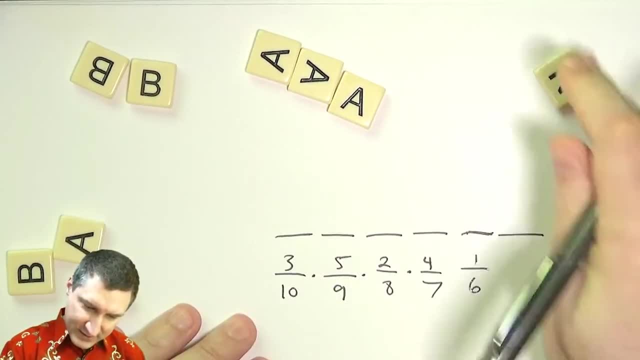 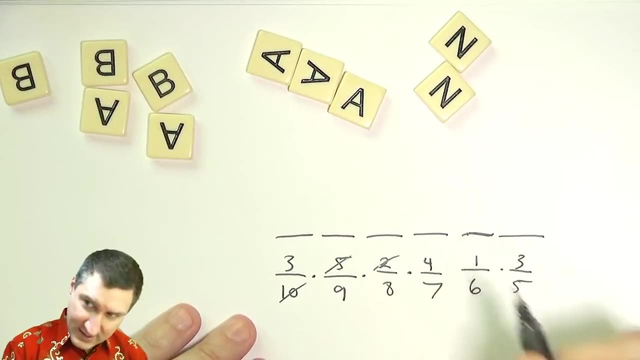 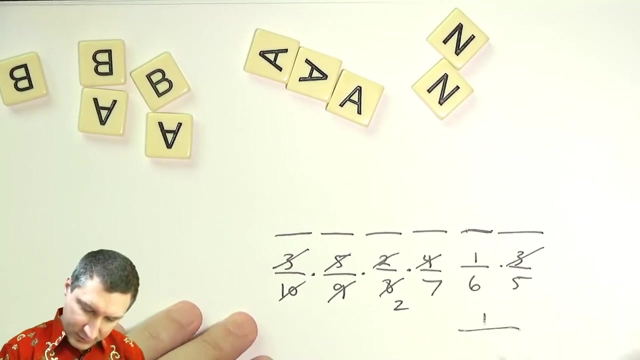 so there's four out of seven. Then I need to pick the other, N, which is one out of six, and then I need to pick another A, which is three out of five, And so now I can do a bunch of things and I can find that what I have left is one over 420, right, That's the probability that. 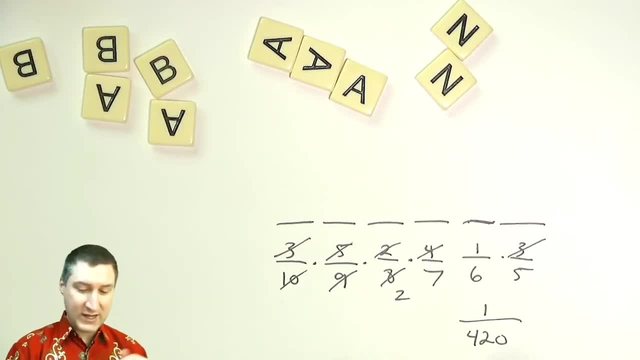 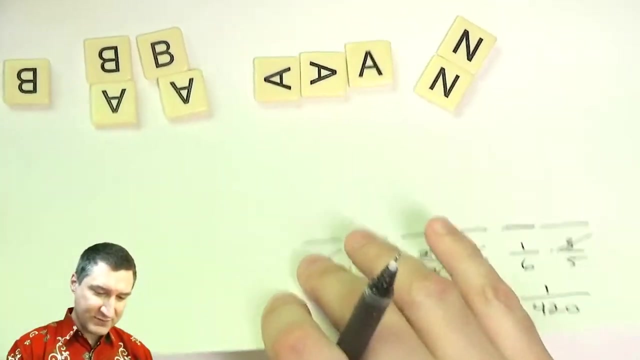 in order. I spell out banana. So now I want to know what happens if the monkey grabs a handful of six tiles out of the bag. Can those tiles be rearranged to spell banana? okay, What's the probability that a draw of six tiles can be rearranged to spell banana? So now we have to do. 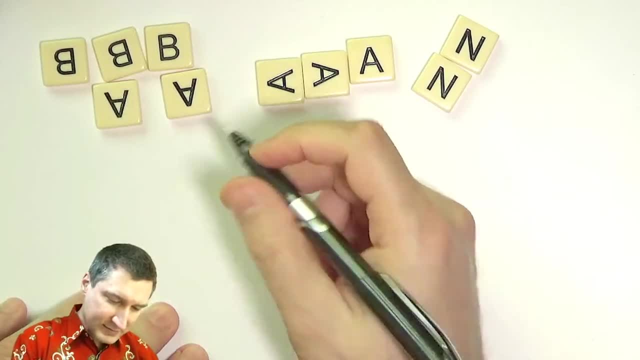 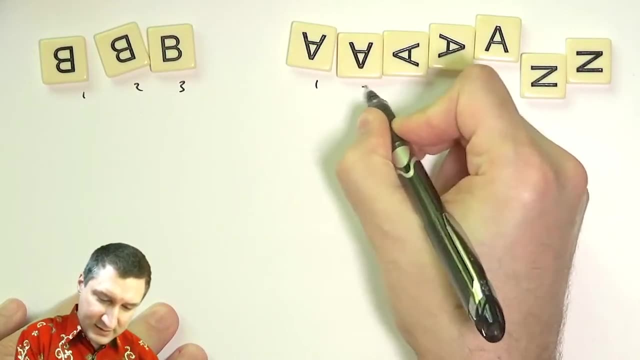 a slight different computation, right? So let's suppose that these tiles are actually numbered, okay. So let's suppose I've got B: 1, 2, 3, A 1, 2, 3, 4, 5, and 1 and 2, okay. So in this, 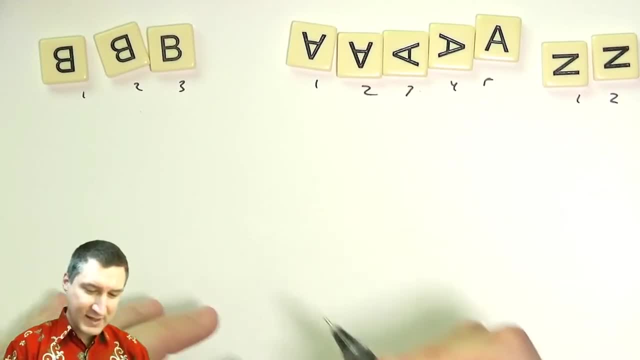 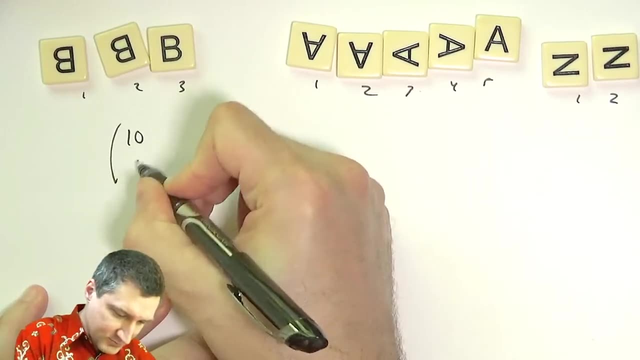 case, imagine that these actually have some numbers to them. Now I'm going to choose six of these 10 tiles. So how many possible draws are there? There's 10. choose six possibilities. and what's that number? 10 times 9 times, 8 times 7.. 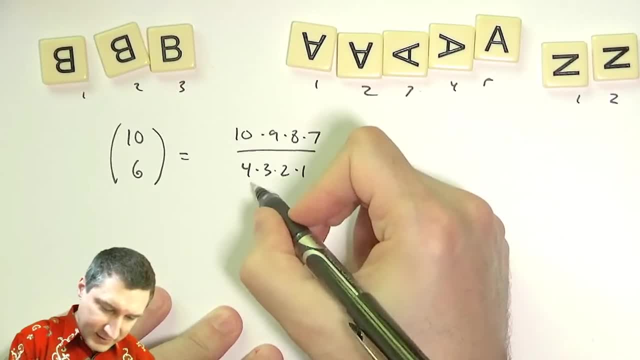 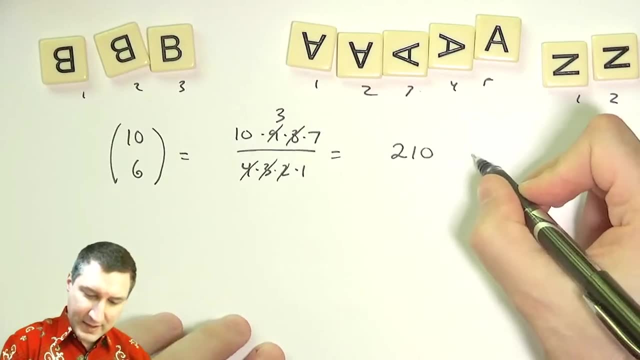 Over 4 times, 3 times 2 times 1.. Again, doing some cancellation, I can get rid of this and I can get rid of this. So I see there's 210 possible collections, assuming that I kind of preserve these numbers along with me. 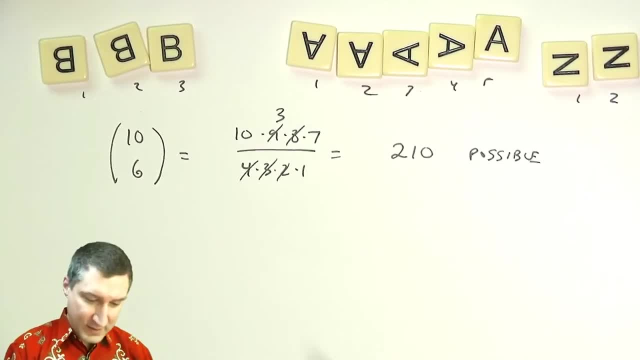 Or now I have to look at how many good outcomes are there, right? So of these, well, I have to choose one of these three B's, So there's three. choose one ways to get the B. I have to choose three out of these five A's, So there's five. choose three ways to get the A's. 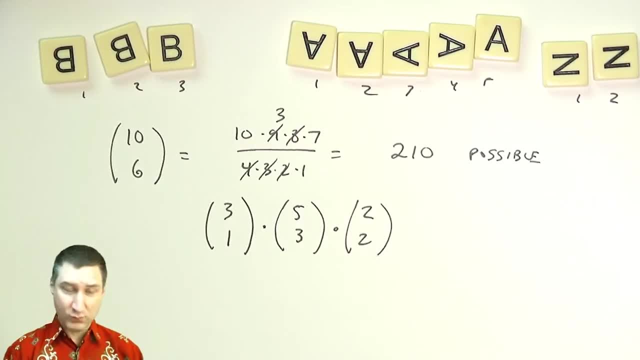 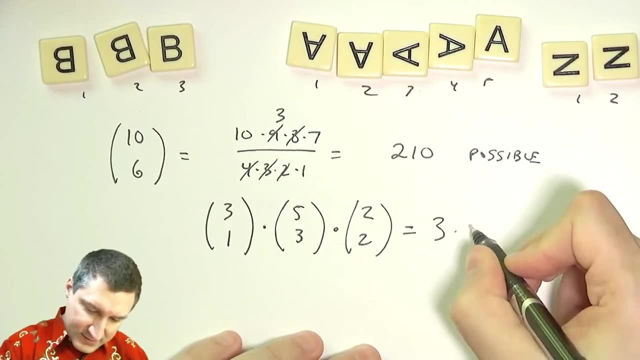 And then I have to choose two out of two N's, Like I have to get exactly one. There's only one way to get the two N's: I have to pick them both out of the bag, right? So now I can compute that the number of good outcomes is 3 times 5, 2, 3 is 10, times 1.. 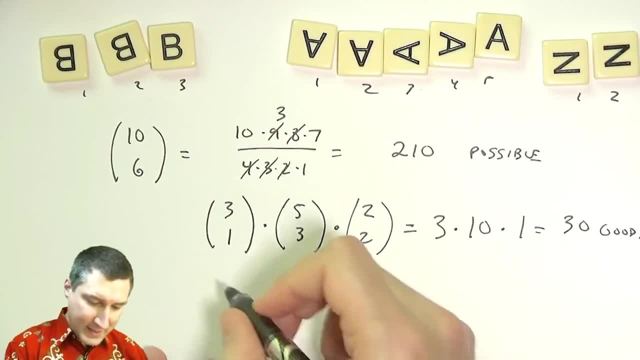 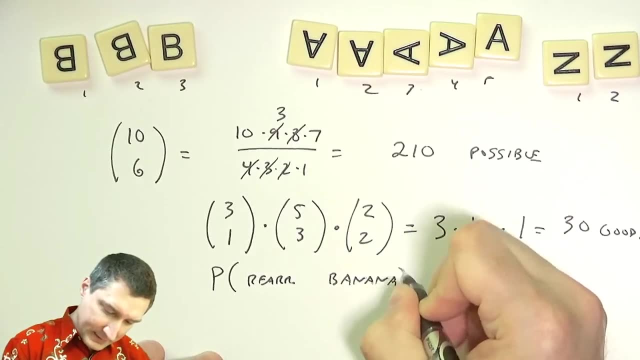 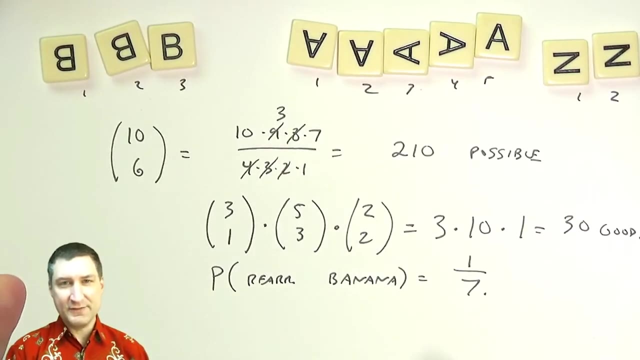 So there's 30 good outcomes And that means the probability of being able to rearrange to spell banana is 30 over 210 is 1 7th. okay, There's a slightly different way of thinking about this. I could think about this and say, okay, suppose that the monkey picked banana out of the bag. 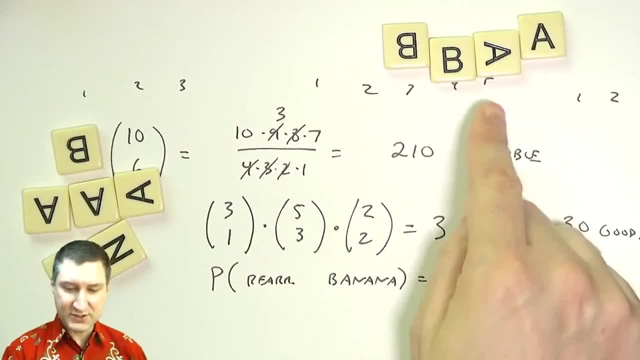 right, What's left in the bag has to be two A's and two B's, And so I can ask myself: okay, how many ways are there to leave two A's and two B's left in the bag? Thinking about that way, 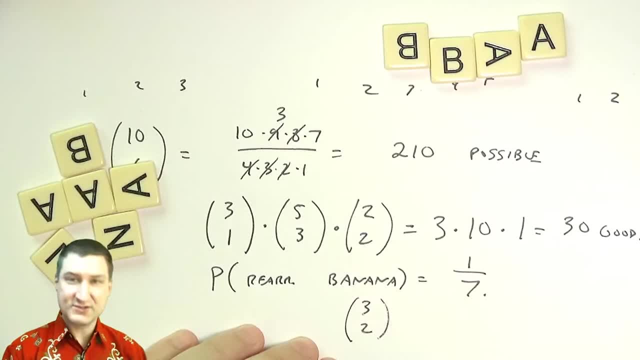 that's like saying: well, there's three, choose two ways to leave two B's in the bag and five, choose two ways to leave two A's in the bag, and three. choose two is three and five, choose two is 10.. So here again, there's 30 good ways. 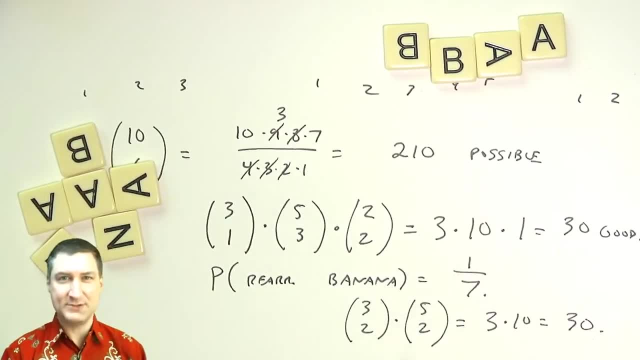 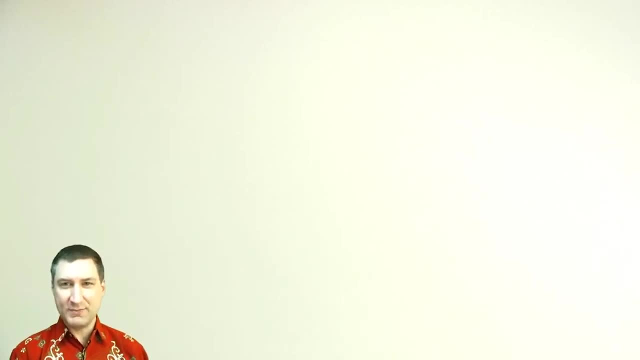 to leave this in the bag So I can do this in a different way and get the same answer. Okay, so that's one example. Another example is: let's go back to the, the classic Avengers. okay, So the Avengers are posing dramatically for a movie poster and I want to know: 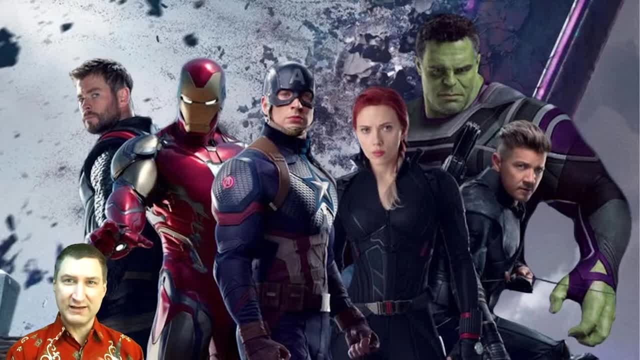 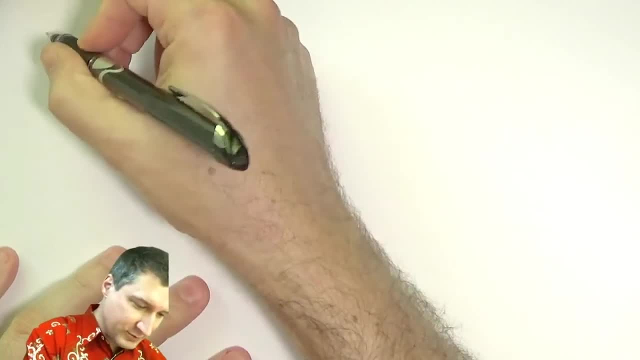 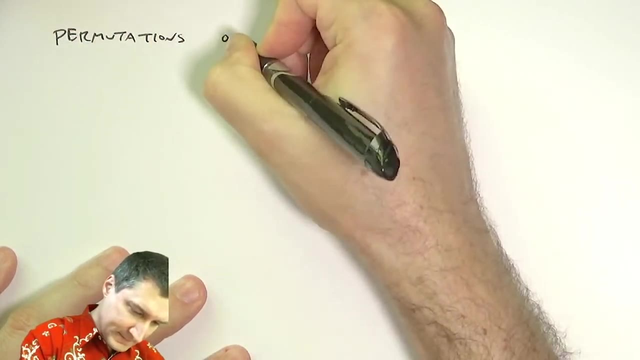 how many different ways are there for these six people to line up left to right? So this is a case where it's a question of how many permutations are there of six people, And that's pretty easy. We know that there are permutations of six people. is six factorial, which is six times, four times? 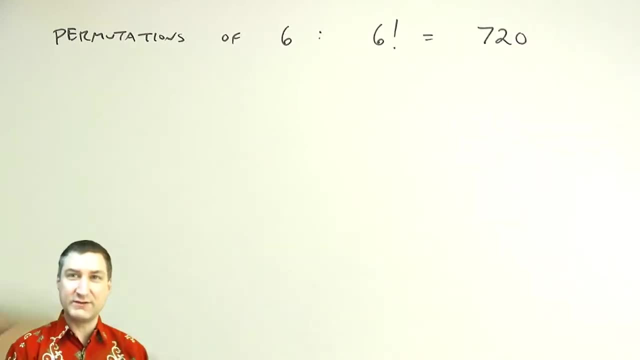 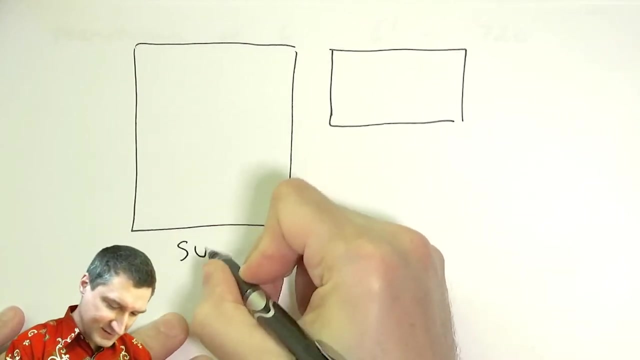 three times, two times one, That's 720.. So there's 720 possible ways that they can line up where order matters. okay, now let's suppose that the Avengers are going to a big battle in two cars. right, there's an SUV that can fit four people and there's a 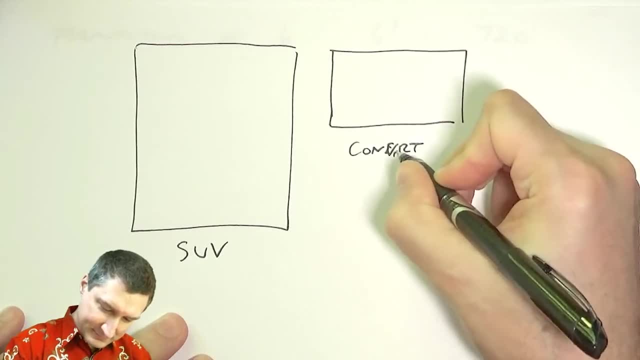 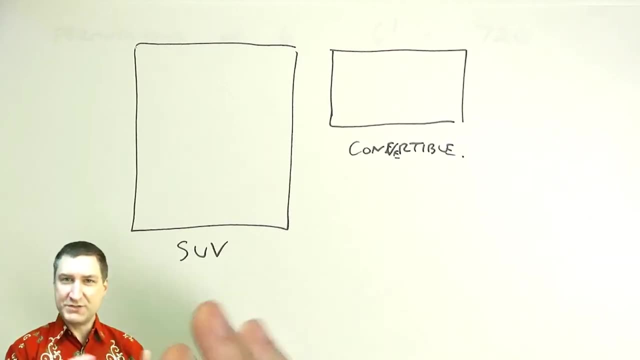 convertible that can fit two people, okay, and I want to know how many possibilities are there for which people choosing. you know which which people are in the SUV and which people are in the convertible, right. so again, order doesn't matter, I just want to know you know how many different ways are there to put. 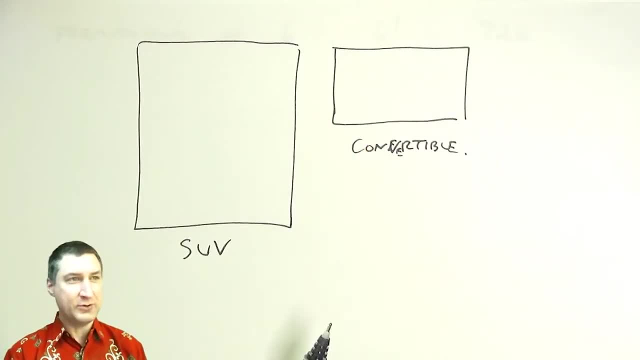 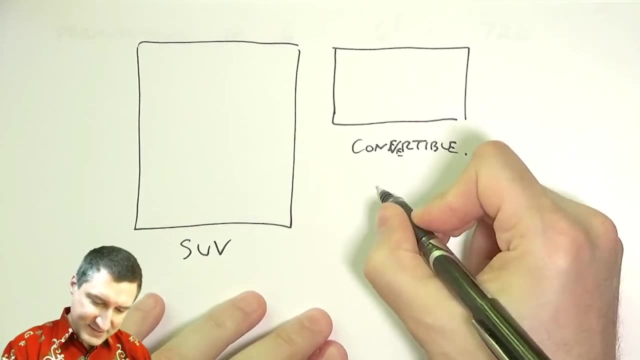 four people here and six people here or it doesn't matter. and so this is kind of like you know n choose K kind of problem where I say, okay, I've got six objects and I could imagine that, okay, I just want to choose which to go in the. 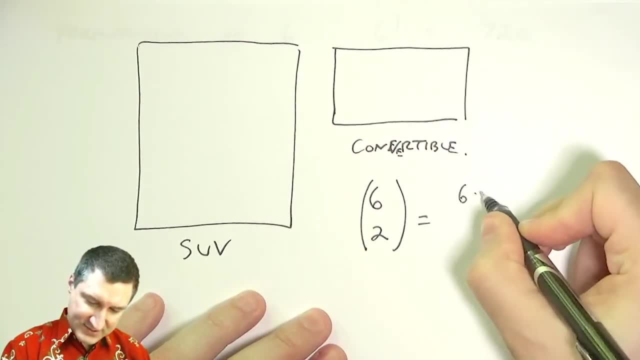 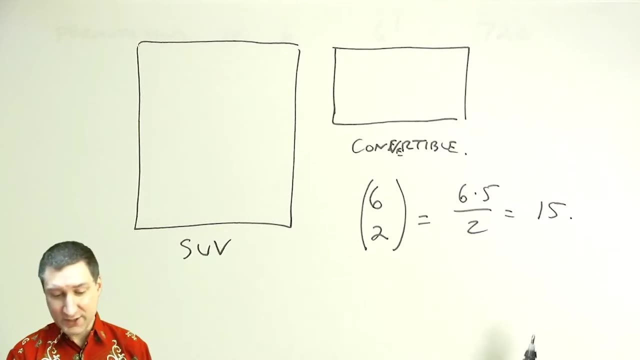 convertible and that's 6 choose 2, which is 6 times 5 over 2, which is 15. so there are 15 possible ways of doing it. you could also, you could also argue- well, you could have just looked at 6 choose 4, right, well, 6 choose 4 is. 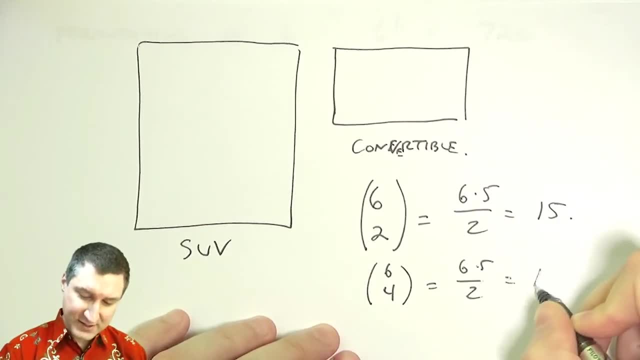 also the same thing. there's this kind of symmetry to the combinatorial, so actually it doesn't really matter. okay, so now I want to know, assuming that each of these 15 possibilities is equally likely, what's the probability that the three cool Avengers out of the six are in the car? so I guess you can argue. 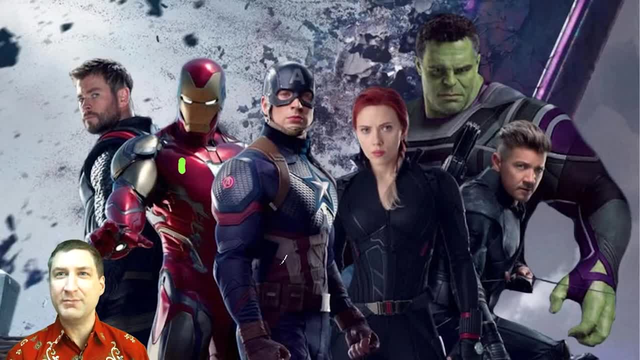 about who are the the cool Avengers? well, Iron Man is definitely cool, Black Widow is cool, Hawkeye is really not cool, Captain America is nice but he's not cool, and I guess we have to decide. you know, Thor used to be lame and now he's cool. and Hulk used to be cool, now he's. 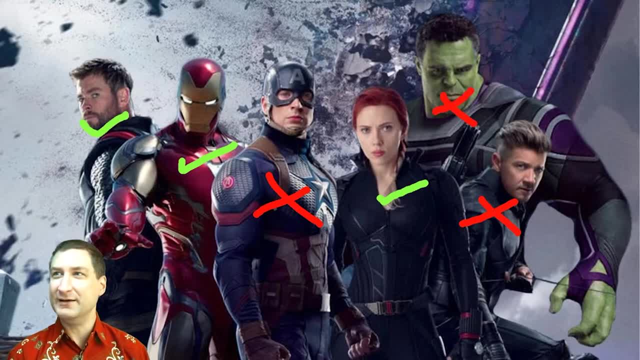 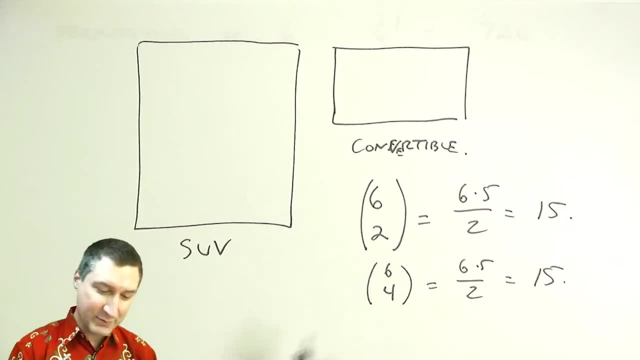 lame. I'm gonna say that Thor is cool and Hulk is not. so we got three good Avengers and three or three cool Avengers and three uncool Avengers. okay, and I want to know what's the probability that the cool ones are all in the same car. so 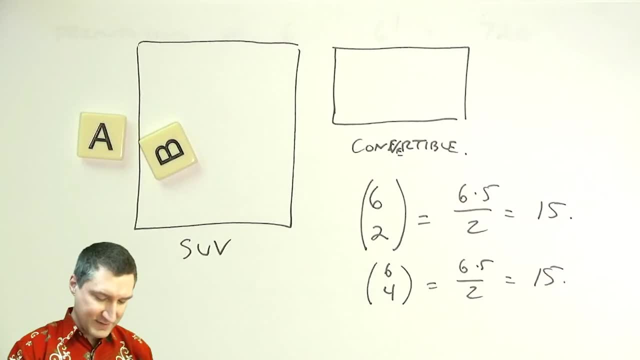 you can substitute what you like for cool and uncool. what suppose that we've got three cool ones and three lame ones. okay, so here I can say actually, well, if I want the three cool ones to be in the same car, the only way that can happen is. 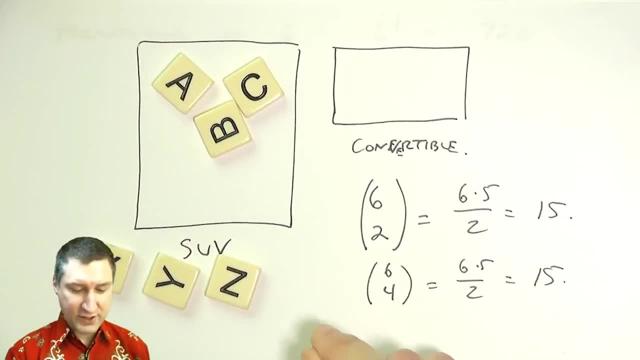 that they're in the SUV, and so that means I have to have three in one car. and then there are only three possible ways that I could have a fourth person in the car. so there are three good outcomes divided by 15 possible outcomes. so the probability- 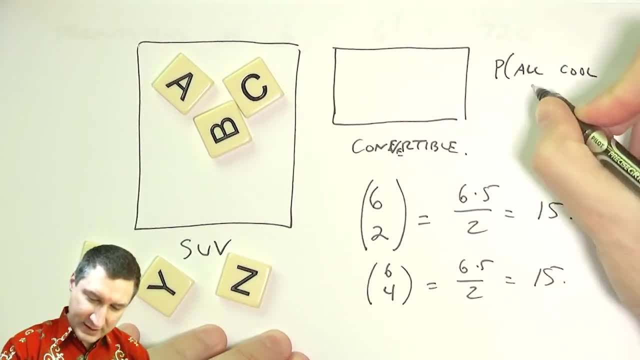 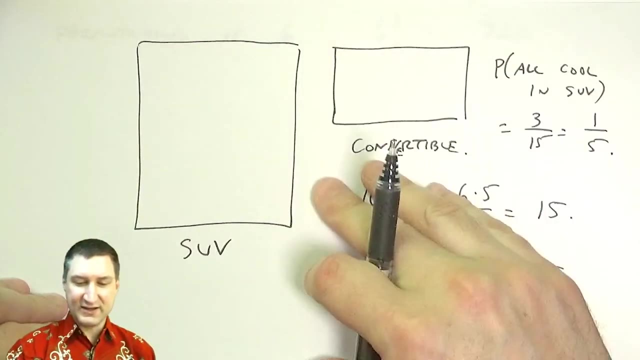 that you know all cool ones are in the SUV is 3 out of 15, or 1, 5th, Okay. so now let's suppose that I switch it up and I say, okay, suppose that instead of going to the battle in the 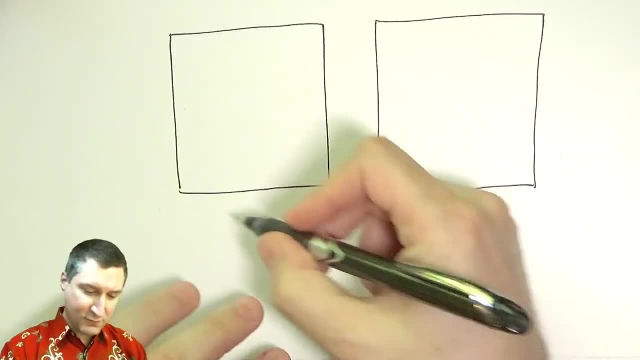 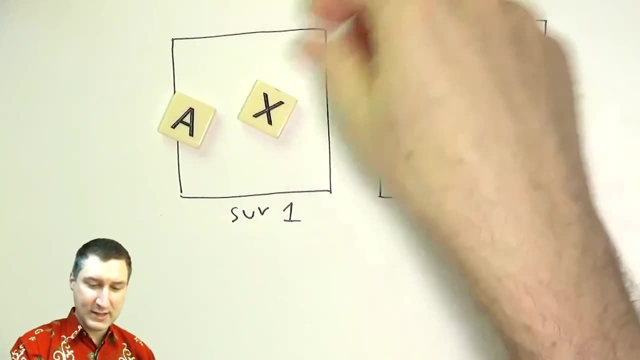 SUV in the convertible. I have two 4-seat SUVs: SUV 1 and SUV 2.. Okay, so that means that, no matter what happens, there's going to be a couple of seats left over right. Let's represent those. 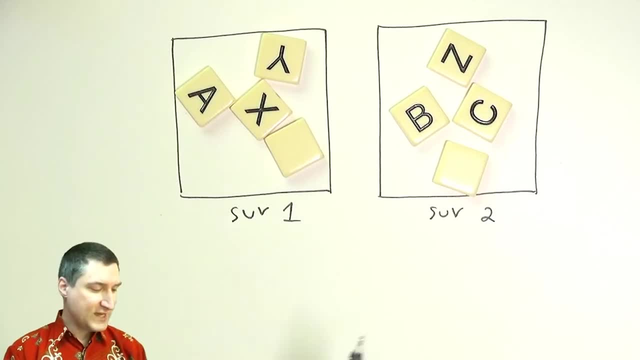 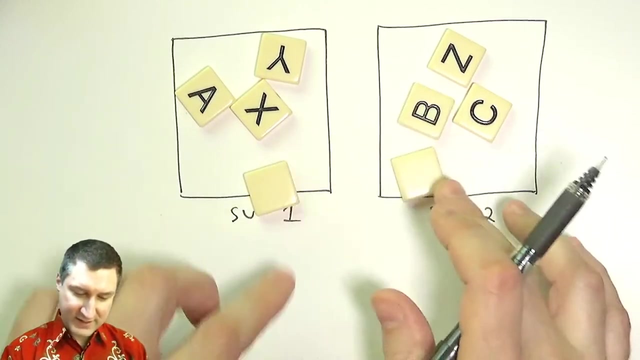 by blanks. Okay, so the first thing I want to know is: how many possibilities are there for who is in what car? Same problem as before, except now I have a couple of extra blanks to worry about. Okay, so these blanks are not distinguishable. right, Those empty seats, And there also could be a little bit. 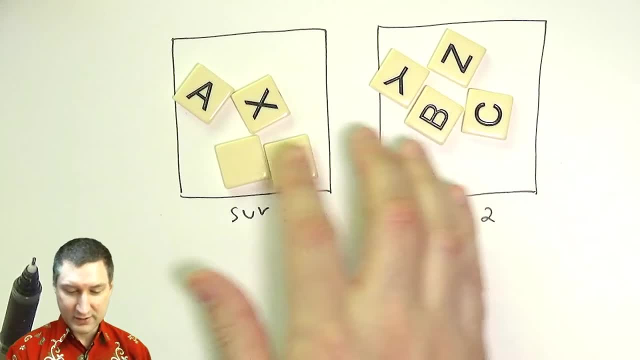 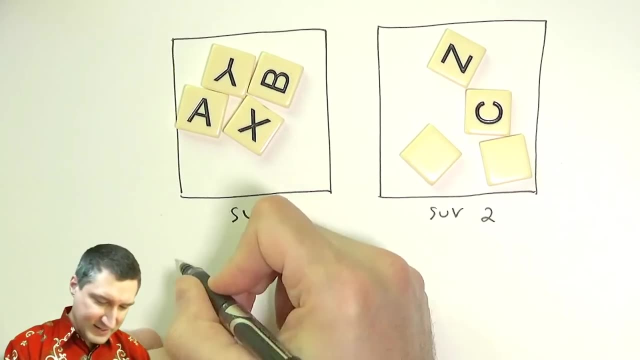 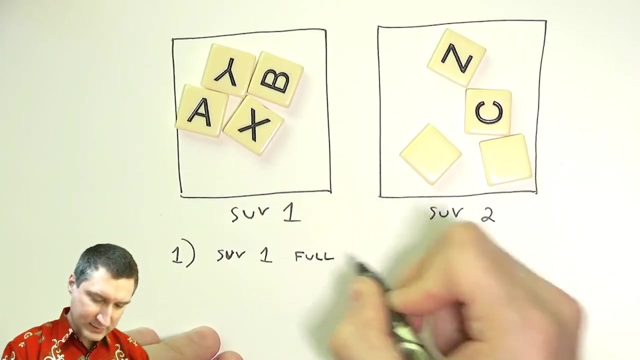 of complication in the fact that two blanks could be in one car or they could be in the other car, right? So we have to kind of look at all the different possibilities. So there are three cases, right. Case one is that SUV 1 is full. Case two is that SUV 2 is full. And case three is that 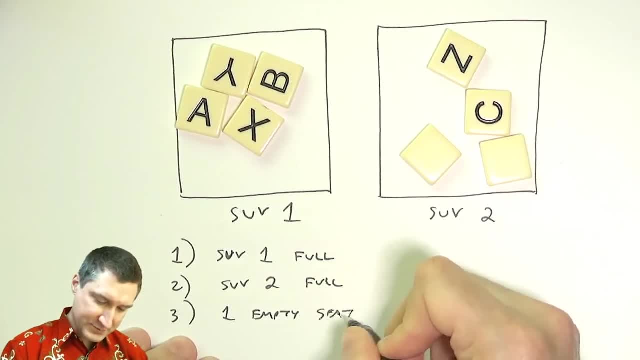 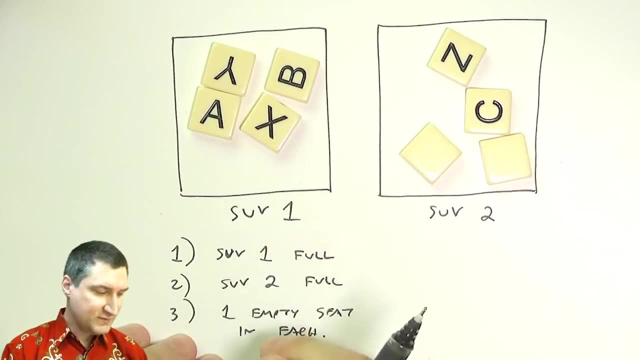 there's one empty seat in each. So let's enumerate those possibilities. How many ways are there for SUV 1 to be full? Well, from before there's six. choose four ways. I have to choose four people to put in SUV 1, and that number is 15.. Same way over here. If I want SUV 2 to be full, there are 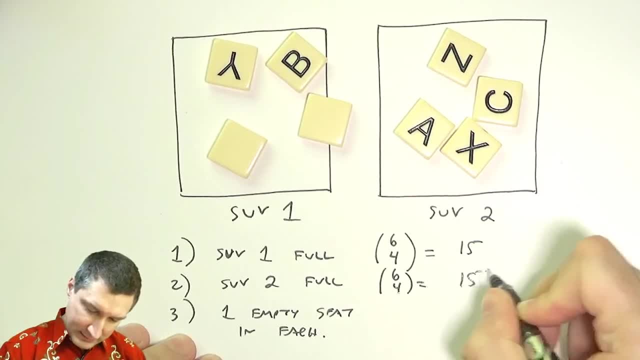 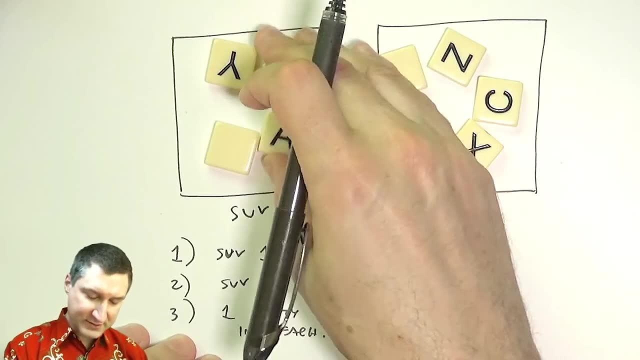 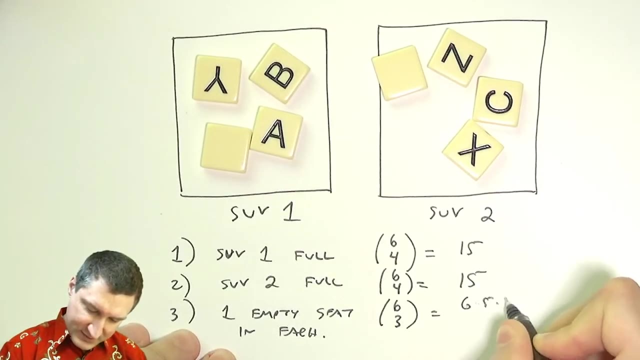 six. choose four ways to make that happen. And then one empty slot in each is more like this: Here there are basically, let's choose the three people in SUV 1. There's six. choose three possibilities there. That's six times four times three. 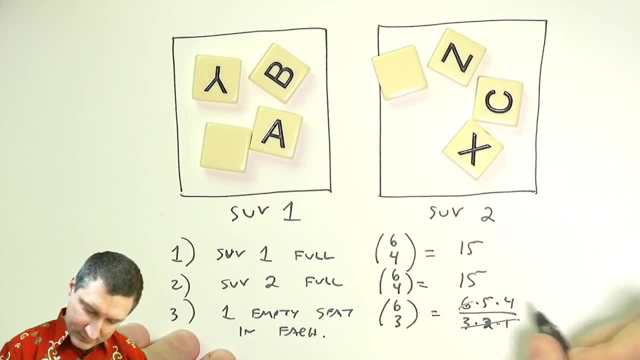 I mean six times, five times four, over three times two times one. So there are 20 possibilities. So overall there are 50 possible ways things can happen. Okay, and now I have to ask: what's the probability that A, B, C are all on the same?